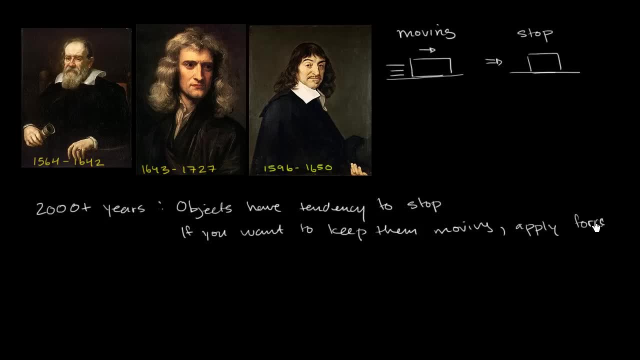 Apply force And once again, this is completely consistent with everyday human experience. This is what we've all experienced our entire lives. But then these gentlemen. this is what Newton showed up in the 1600s, And you might be surprised to see three gentlemen pictured here. 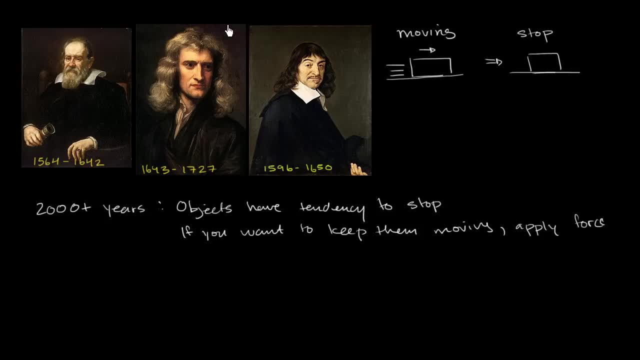 because this was about Newton's first law of motion- And indeed one of these gentlemen is Sir Isaac Newton, That's Newton right over there, But these other two guys get at least as much credit for it- because they actually described really what Newton's first law describes. 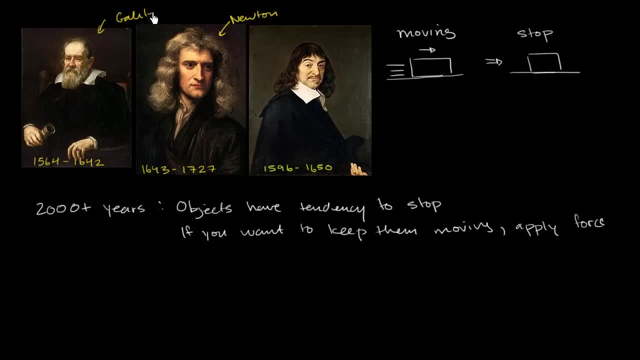 and they did it before Newton. This is Galileo Galilei and this is Rene Descartes, And they described it in different ways And Newton frankly gets the credit for it because he really encapsulated it into a broader framework. 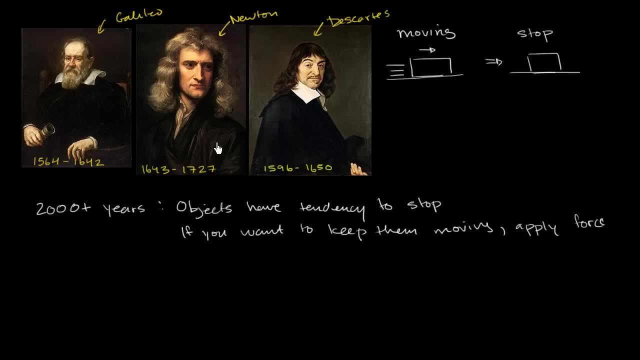 with his other laws and the laws of gravitation, which was really the basis of classical mechanics and seemed to describe, at least until the 20th century, most of how reality actually worked, And their big insight, and it was very unintuitive at the time. 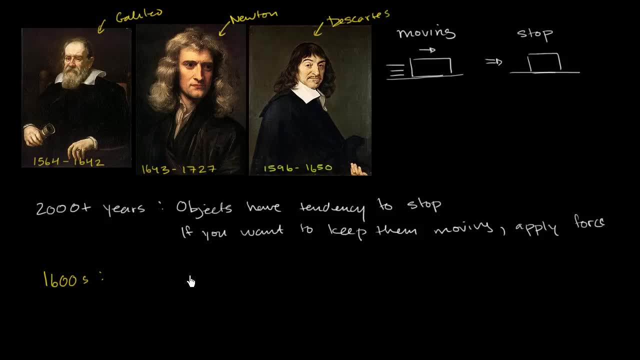 so now we come to the 1600s. is that these three gentlemen said? maybe it works the other way? Maybe objects have a tendency, have a tendency to maintain, to maintain, maintain their velocity, so their speed and their direction Have a tendency to maintain their velocity. 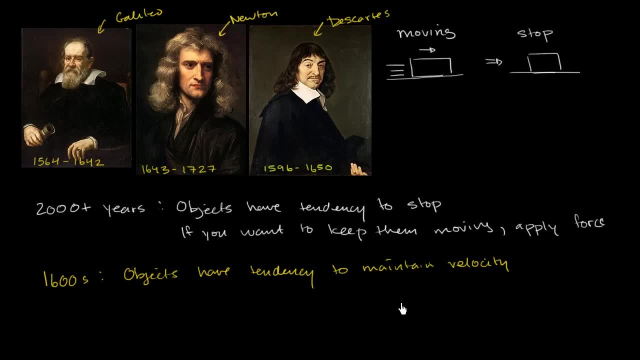 and if their speed is zero, they'll maintain that restfulness unless they're acted on by an unbalanced force, Unless unless acted on by unbalanced, unbalanced force, Unbalanced force. So completely the opposite way of thinking For 2000 years. objects tend to stop on their own. 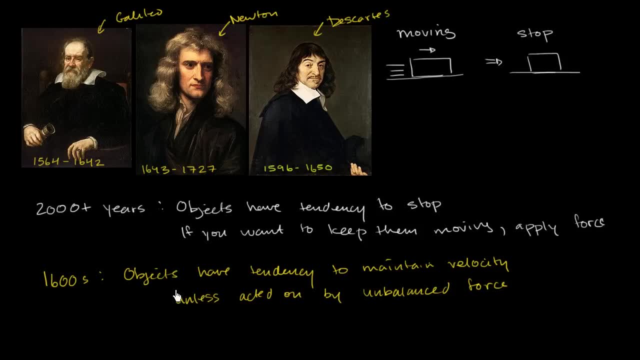 If you want to keep them moving, apply a force. These guys say. objects have a tendency to maintain their motion forever and the only way that you're going to stop them is if you act or accelerate them or change their velocity. so either their speed or direction some way. 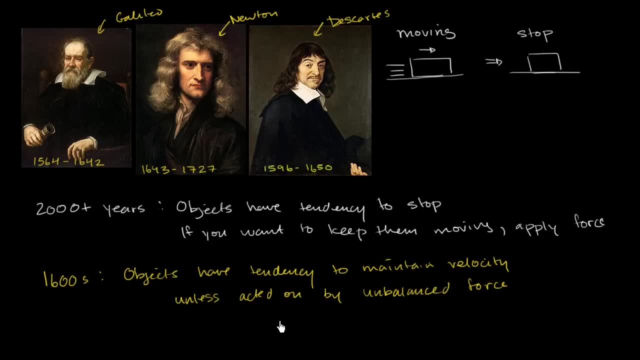 is to act on them with an unbalanced force. But you might be saying, hey, come on, Sal, what's going on? You just went through this. you said: for most of human history, including my own personal history, this is what I observed. 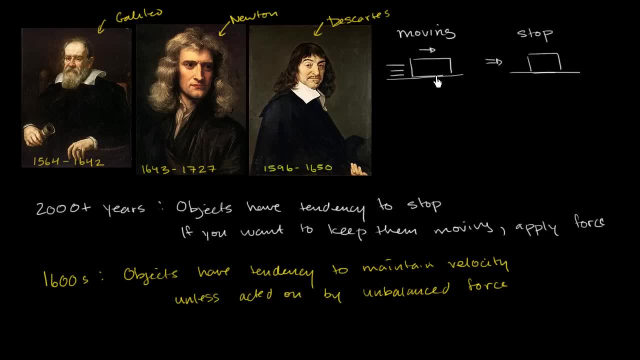 How can these guys say that this thing has a tendency to go on forever? This seems to break down, And their big insight was: well, maybe these things don't have by themselves a tendency to stop, but because of interactions with their environment. 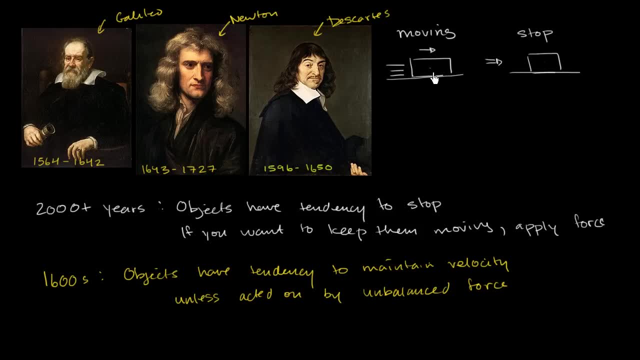 forces are being generated that are acting against their motion. So when you think you're just leaving this thing alone, there's actually a net force that is trying to stop it, And this particular example right over here, this net force, the net force, is the force of friction. 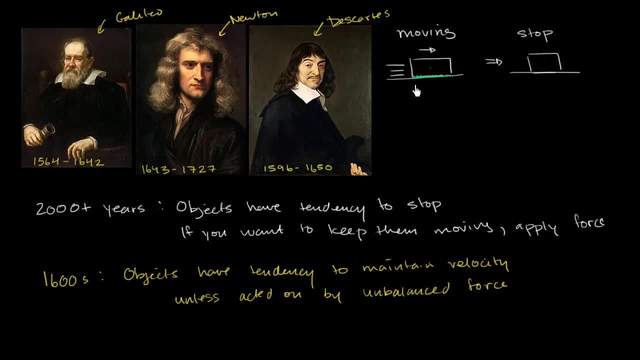 It's the interaction between the block and the ground. So this thing, when you think that you're leaving this thing alone, you actually have a net force that is going against its motion, which is the force of friction, And these guys realized that. 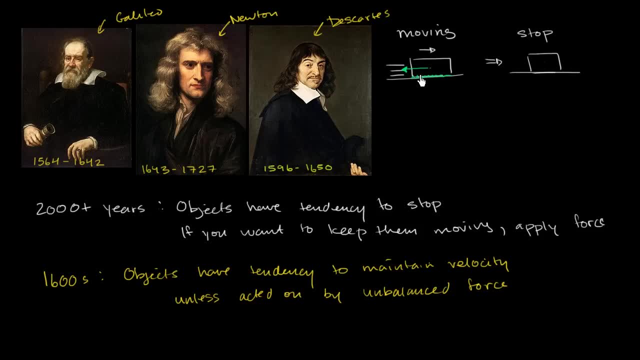 because they said, look, if it was an innate property of the block, regardless of the environment, it should kind of always come to a stop in maybe a similar way. But they saw, if you made this surface a little bit smoother and a little bit smoother, 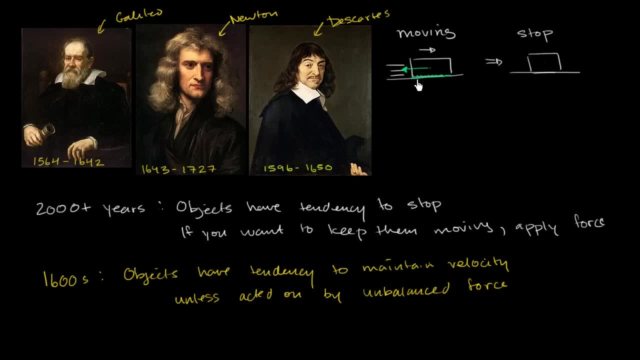 this thing would travel further and further And maybe, if you eliminated this friction, this made the surface completely frictionless, completely smooth. this thing, indeed, would travel forever, And they didn't have the luxury of launching satellites and doing things in deep space. 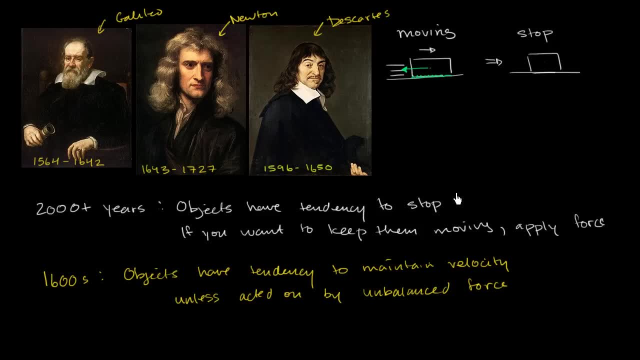 So it was a very, very, very unintuitive thought experiment. And then you might say: well, what about this other thing? What happens when I am applying a force? Because in my everyday life, if I want to drag my TV set across the room, 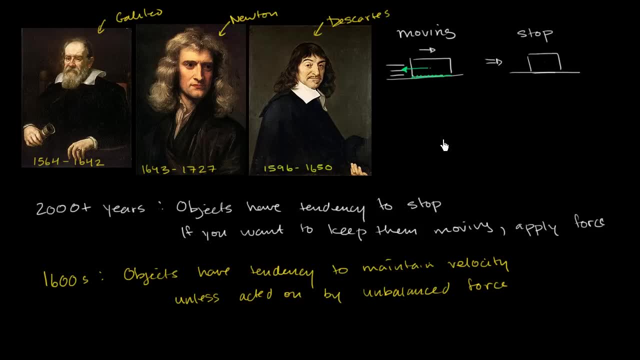 I apply a force to it And what these guys would tell you is all you were doing if you were keeping the velocity of that TV constant. all you were doing was counteracting this net negative force. So if this was a TV dragging across your carpet, 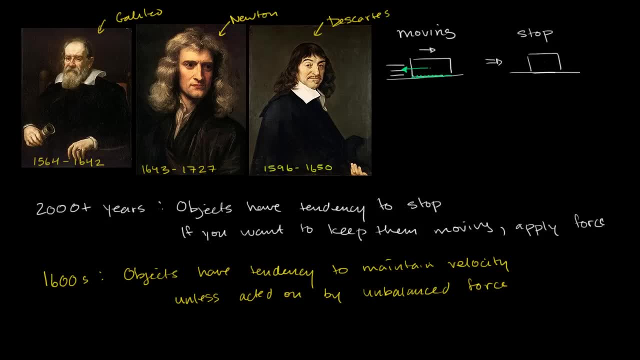 this is the force of friction acting against the motion of the object, And so you are essentially just balancing it when you push it. If you balance it perfectly, you will be able to maintain its velocity. If you want to accelerate it, you will have to apply even more force. 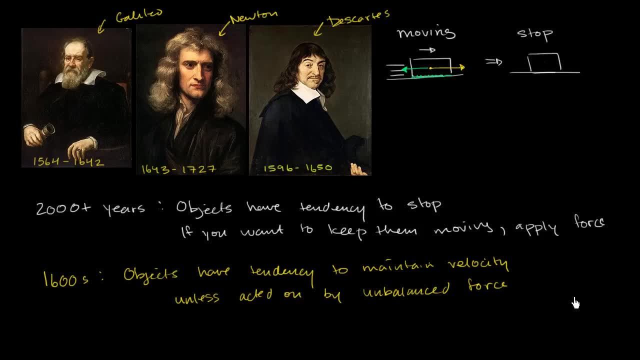 in the direction that you are acting. You are actually pushing it.